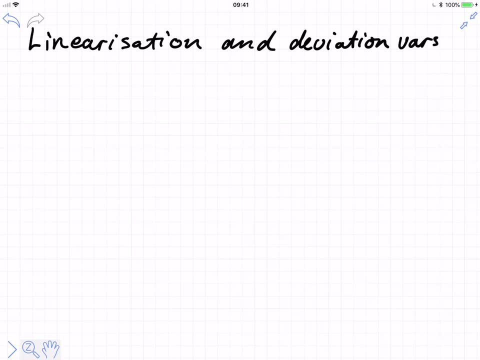 that are difficult to explain and difficult to understand. The solution of nonlinear differential equations is a very complicated topic. It can get very difficult, very quickly. differential equations in an analytic form is still an active topic of research and we are not 100% sure whether it is possible in general to solve any of the differential 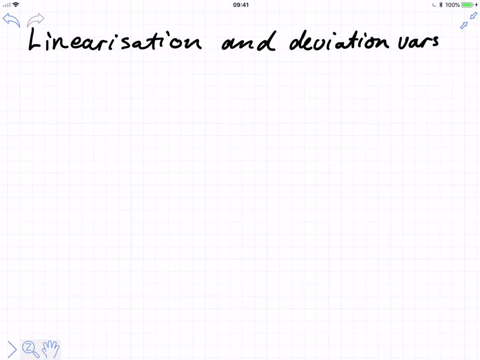 equations that we just look at because there are no general rules. So it's not like easy. things like polynomials, where we know things, like the fundamental theorem of algebra that says: oh yes, well, here's a polynomial, We know that it has solutions, We know that. 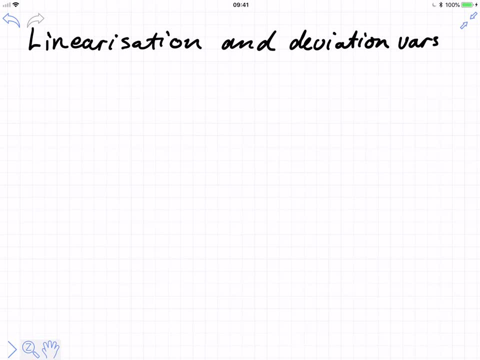 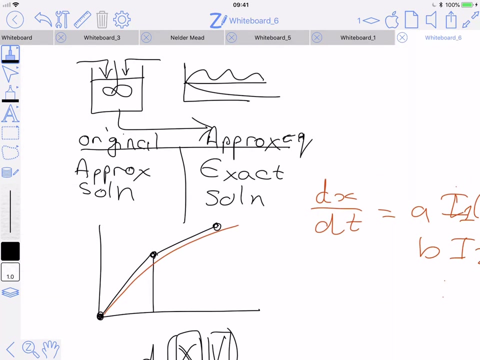 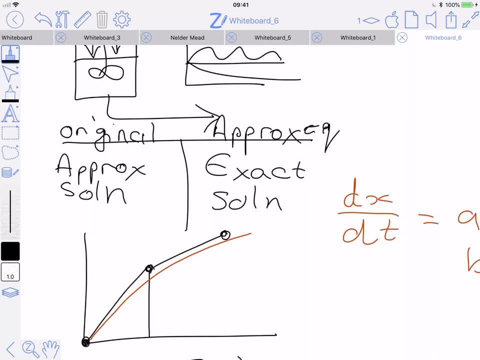 The one approach that we'll be following- and that you already did for TUT3, is to take those equations and then solve them approximately or approximate the solution to the differential equations using numeric methods In class and for the analytic work that we'll be doing, 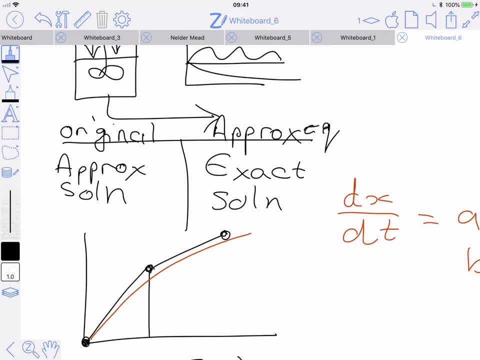 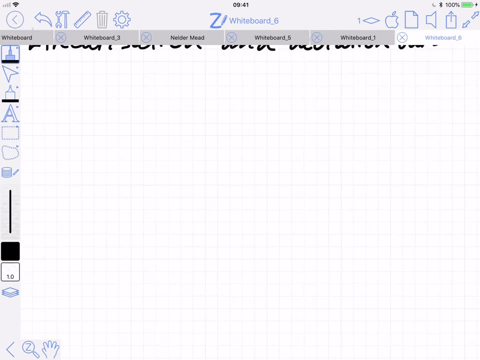 in this subject. we will not be doing that. We will not be using numeric solution, but instead we will be doing analytic solution of approximate equations. And the specific thing that we're going to be doing to approximate these equations is we're going to always approximate all the behavior of the systems as linear differential. 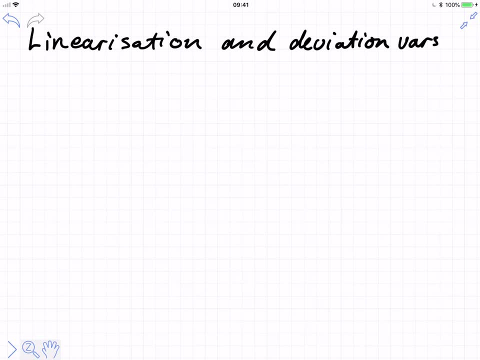 equations. The reason why we do that is because linear differential equations have well-behaved and well-known solutions. So we have exact solutions to linear differential equations where we do not have exact solutions. And we have exact solutions to linear differential equations where we do not have exact solutions. And we have exact solutions to linear differential. 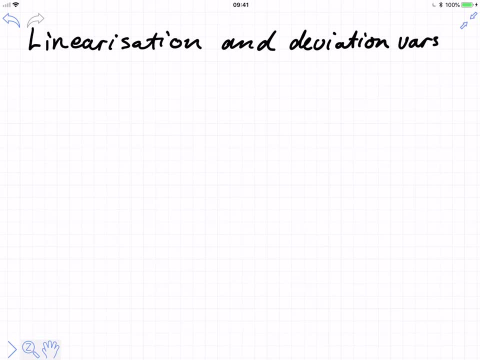 equations. So we're going to proceed through a sequence of steps. Whenever we find a general nonlinear differential equation that we've just developed from writing out the balance equations, all the stuff that we've been doing in the first two TUTs, we're going to look. 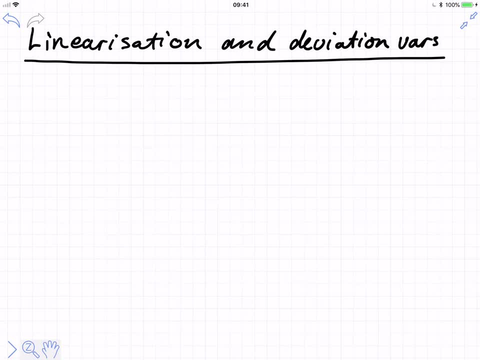 at that equation and we're going to first identify nonlinear terms And nonlinear terms just to explain. a general differential equation looks like that is of linear form. it always will look like this. so this is what a linear differential equation looks like. I've included here this function of time specifically to say that and that that. 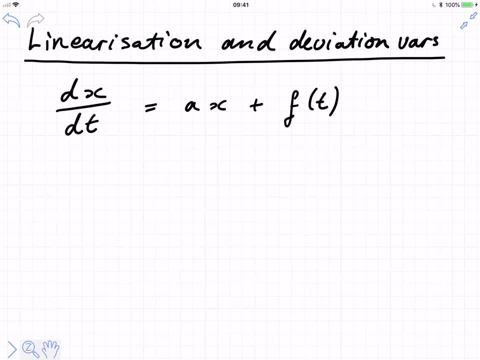 function of time is sometimes called the forcing function. you may have come across this in a mental attribution before. this forcing function is not subject to the same restrictions as the other parts. we're talking about linear participation of the variables that take place, that take part in the equation itself. so in other words here: 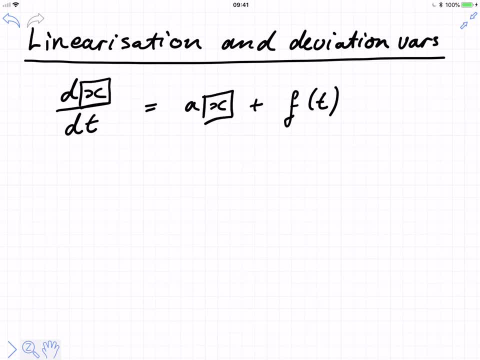 we have a state variable and that state variable is appearing linearly in the input right. this f of T called the forcing function can be any function of time, So that can be sine of time, or it can be log of time, or it can be any kind of weird function of time. 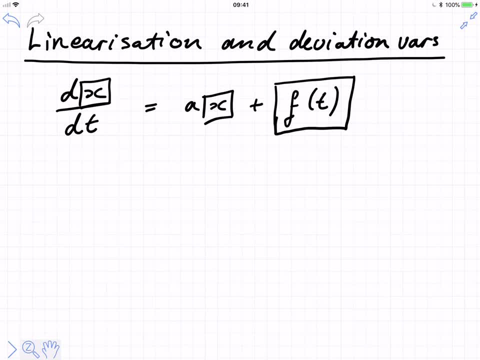 It can be T squared, It can be just what it wants, right? In general, we do not place any linear restrictions on the kind of function of time that we're talking about when we're talking about the forcing function. What we're talking about linearizing is all of the other variables. 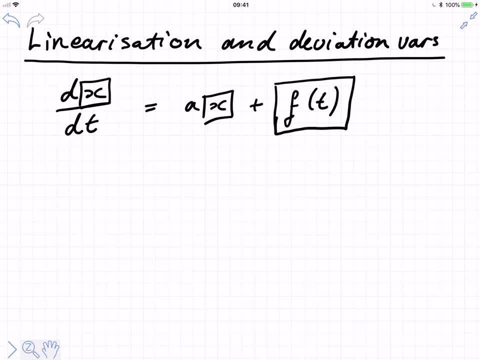 that take part in the actual differential equation itself. Now, this is an important distinction, because you'll see, but also notice, that we don't allow for any, so there can't be like an X here, for instance, right? So the terms in the linear differential equation, 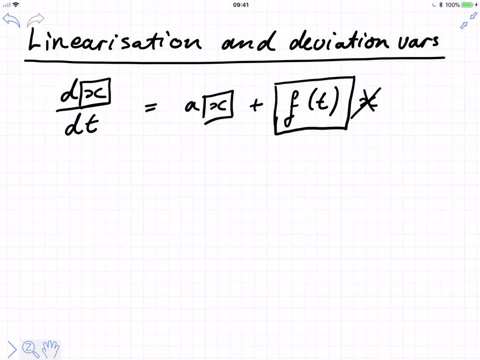 all of the variables, the variables that take part in the differential equation, must appear linearly. Time is an exception, So any formula that is only a function of time, that's perfectly fine. That is part of the forcing function and we don't worry about that. 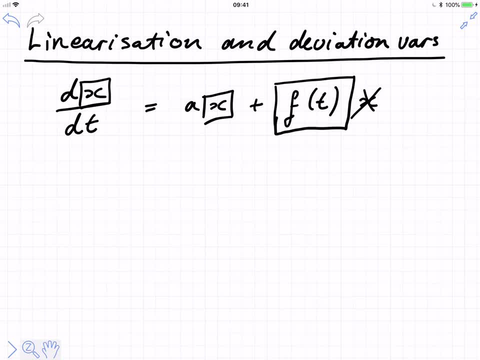 So just be clear that we never attempt to linearize pure functions of time. So if there's a sine of time somewhere, or if it's T squared or anything like that, we will keep that exactly the same. So this is our target form. 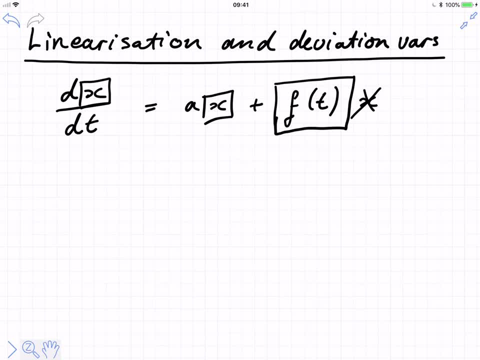 And in general, if we have systems of differential equations, we may add extra variables. So we may have something like this, and this may be something like BY plus CX plus F2 of time, And so here we now have a system of linear differential equations. 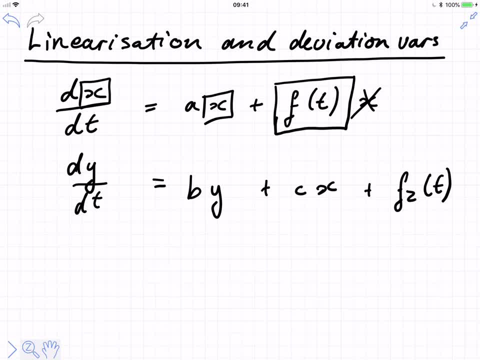 Right. So now we have two differential equations and they are both linear. We know that they are linear because here we have another state variable and both the state variable and the other state variable appear only linearly in these equations. I find it's easier to start, you know, to what they call. 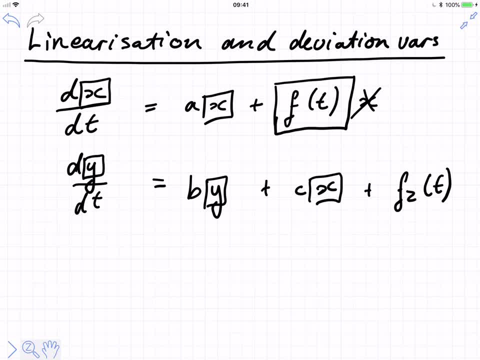 begin with the end in mind, right Where, if we know that this is the target. in other words, I want to take whatever differential equations I have and I want to write it in exactly this form. It becomes a lot easier to do the manipulation. 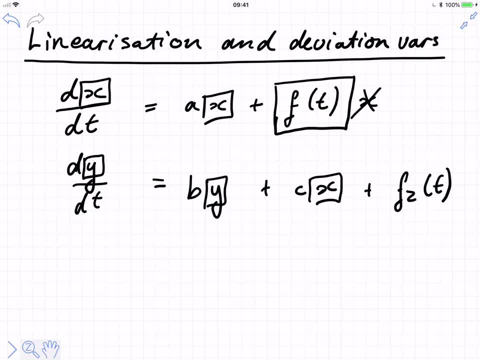 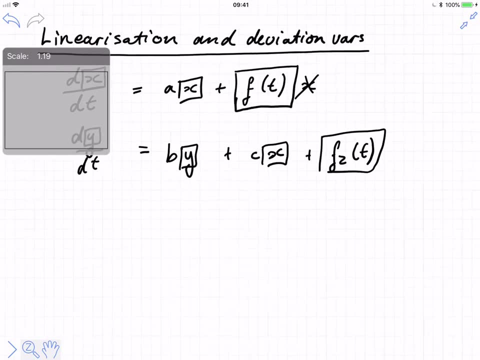 because you know what kind of form you're actually targeting. You're targeting a form where there are constant coefficients multiplied by each one of the state variables. Now you will also see. you will also see a slightly different form of this, which highlights the idea that everything is linear in these equations. 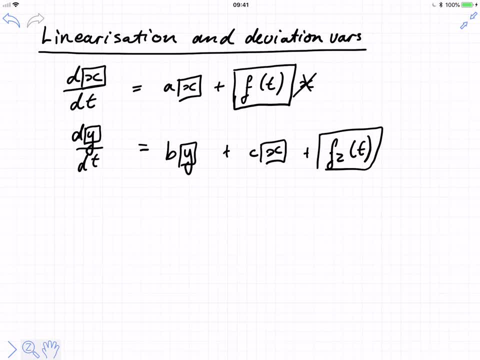 where, where, where, where, where, where you may find these f's of t being replaced by input variables, And so we could say that that's actually just u, maybe u1, and this is u2.. And a relatively standard form for these. 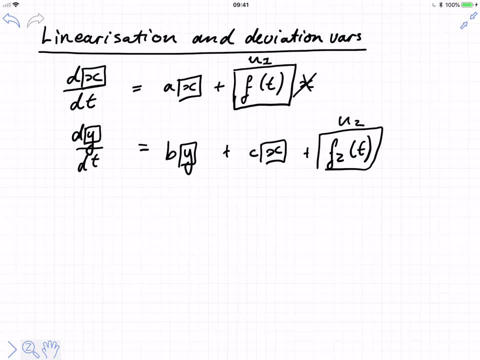 and I've used this. I've just used x and y now, but it is quite standard for us to, for us to to standardize our approach so that we've got x as a vector being all of the input variables, y as a vector being all of the output variables. 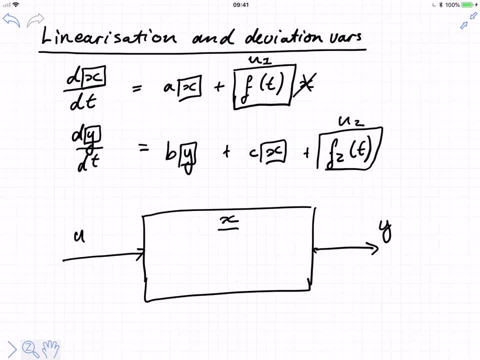 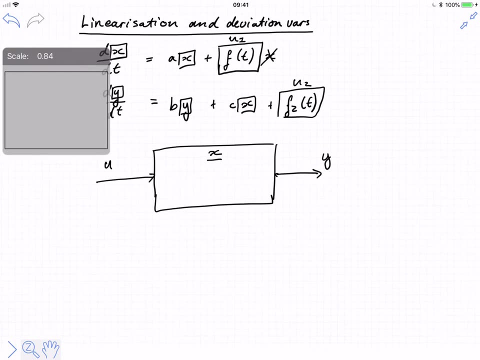 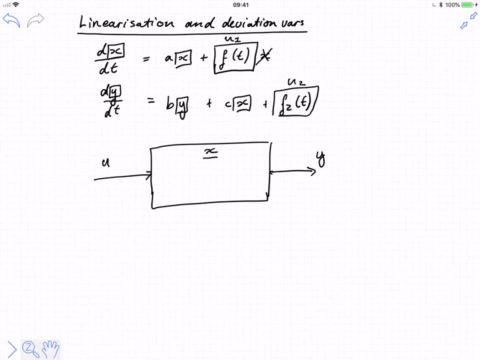 and u being all of the input variables. And you'll see references to this standardized form in tutorial four, which was uploaded onto ClickUp yesterday, where we will actually manipulate this, this form, even further, And in this case I'm going to choose these symbols so that we have a dx vector dt. 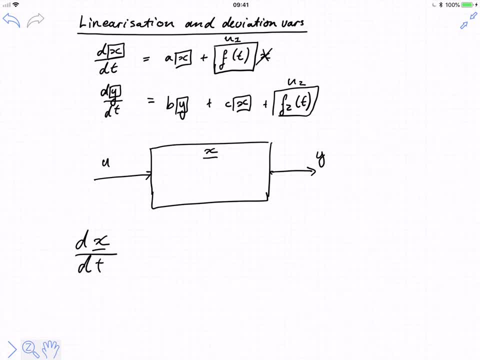 And now notice I'm going to be using kind of vector notation here. So those are both of the left-hand sides and we can say: and let's say that our x vector here, x vector here, is equal to 0. This way, 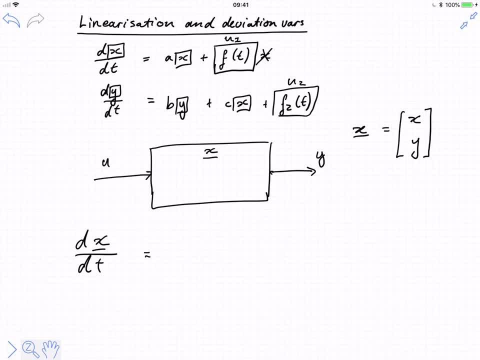 so we can assume, And so that's a control that we can use, And of course those are. so that's a control that we can use. if we choose x, vector y and that vector y is this, vector x y. 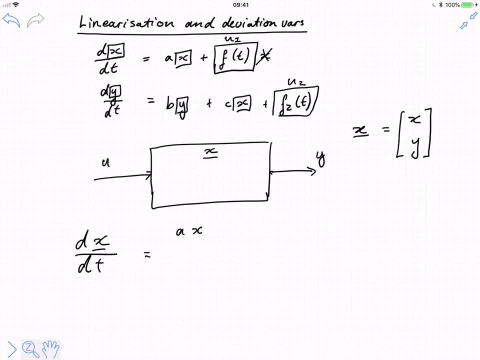 so we have- and I'm going to write this out in long form first and then simplify to array form- where I've got a x, one got a c x1. And I'm just going to apply it. Now you can see that we've got a x1 vector. 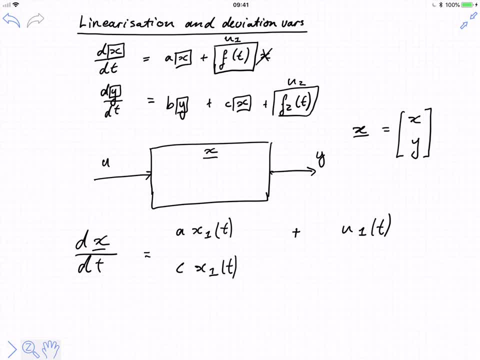 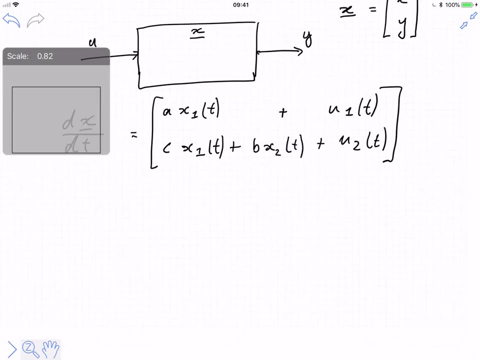 going to also highlight here that these are functions of time. These things change over time. So now I've got this in a vector form. So in other words, I'm just writing both of those two elements of the vector and we can see that that's going to result in a matrix. 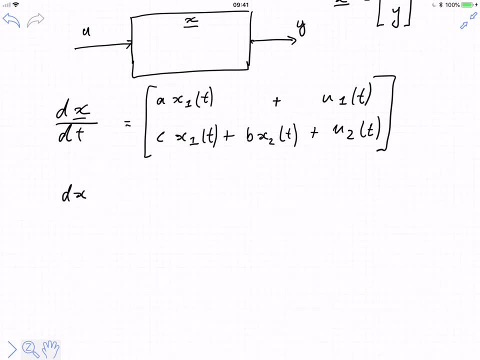 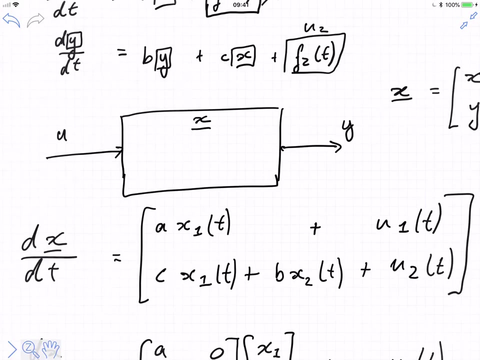 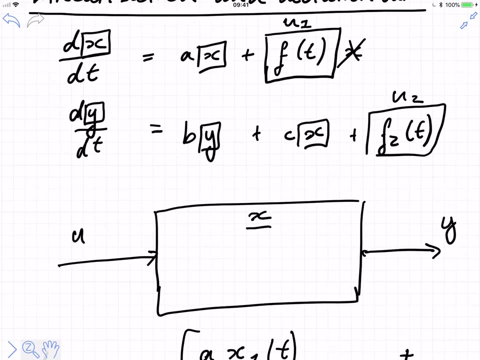 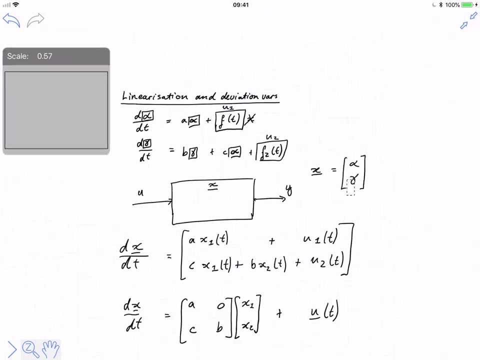 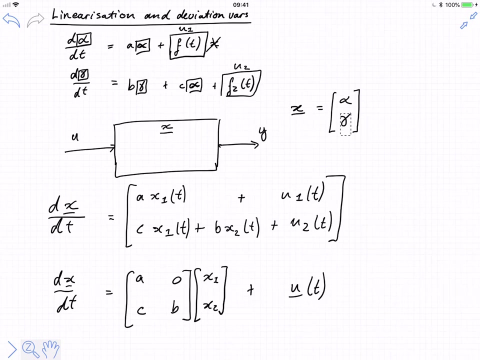 expression where we'll have dx, dt equal to a, 0, c b times x. Maybe it will make it simpler if I just use different symbols instead of x and y. Okay, Does that make everything a lot clearer? Happy, Okay, Don't get confused with symbols. 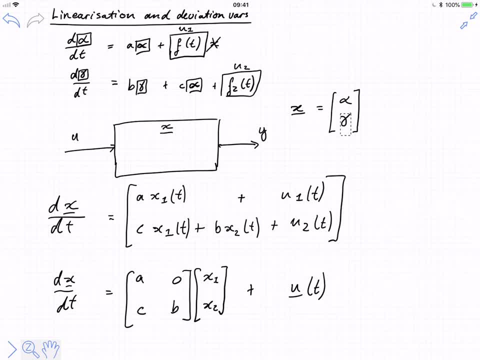 Okay, Don't get confused with symbols, Right, But and don't get too attached to particular symbols once we've kind of done something like this, So okay, So we've got state variables in the model that I wrote down at the top. It was just alpha and gamma, And I've just reworked that so that I have 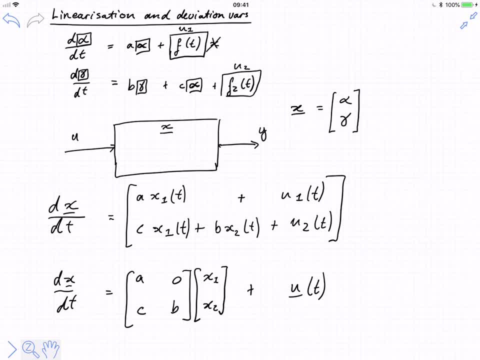 that in a linear form, And by convention, we'll often call this whole matrix here, we'll call that a and there'll be, And we'll often call that b. Okay, And so this is just So. we've got a linear combination. 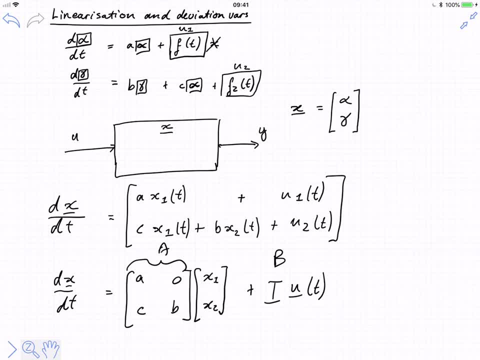 of the states and that linear combination coefficient is a. and we've got a linear combination of inputs and that linear coefficient is b. Now some of the eagle-eyed among you may be thinking: hang on a bit, There's something there. There's something there, There's something. 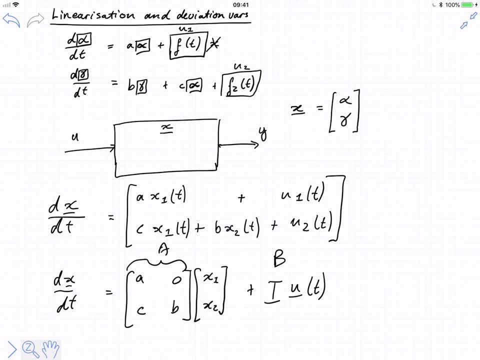 there that is still linear, but which isn't encapsulated within this form, which is- I could add a constant term to any of these equations Right, And those things would then not be. There's no way to combine inputs in a linear way to get one Right If they. 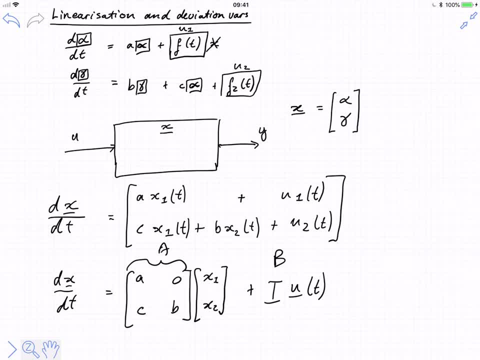 are changing, If u of t or these inputs are changing, I could. I can't combine them. I can't combine them in any way to get one of the constants. So you say, wait, I should make, I should have a space to add a constant. And because we are going to try and make these, 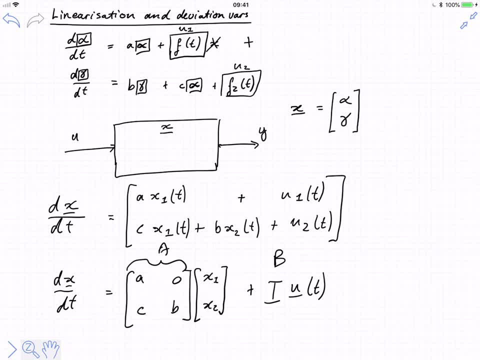 things easy to solve. we are going to take steps to make sure that this constant will always be zero, And the steps that we take to do that is, we will shift our axes. We will make use of different variables called deviation variables, And those deviation variables are chosen, such: 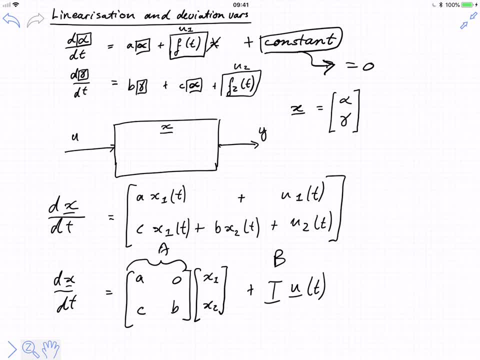 that their initial values are equal to zero. So, on the one hand, this is our target: We're trying to massage or approximate every possible interaction of variables In this linear way, And we're going to try to approximate that in such a way so that 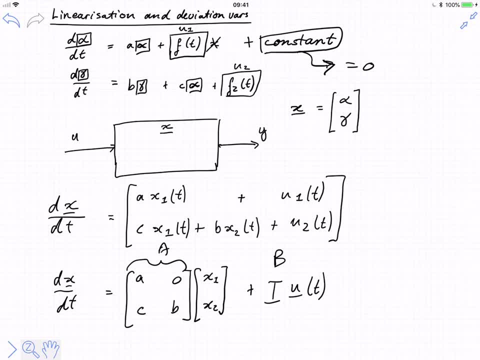 not only do we only have a linear combination of variables leading to every single differential equation, so that we don't have any non-linear terms. Remember, barring functions, pure functions of time are allowed to be themselves. We never attempt to linearize pure functions of time. 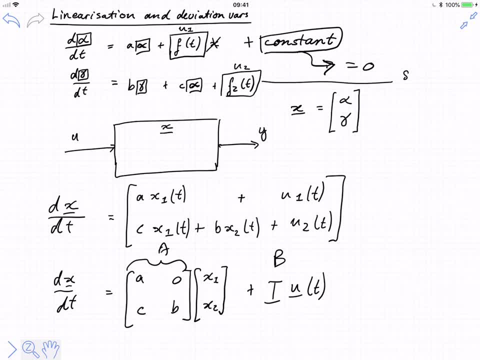 So all of these things, if we see something like sine of t or cos of t, of all of those things we don't approximate only if they are appearing by themselves as forcing functions, So if there's a combination of variables. 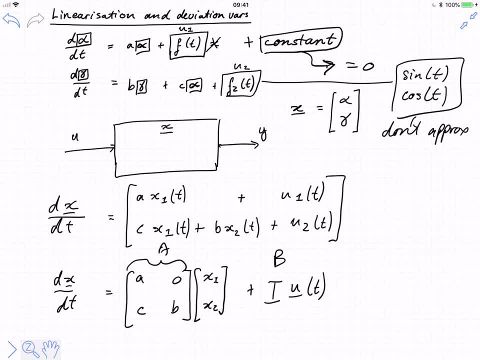 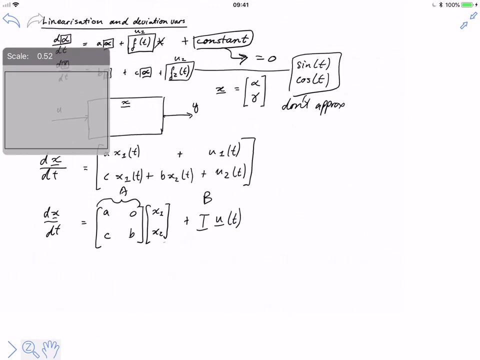 so if that was alpha times, sine of t or anything like that, those multiplications we definitely do linearize. But if we see somewhere in an expression just a pure function of time, we don't try to approximate that at all, The mechanics of this. So this is the goal. I wanted to start with the goal in mind because 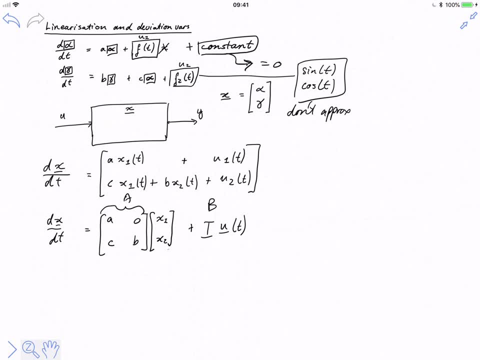 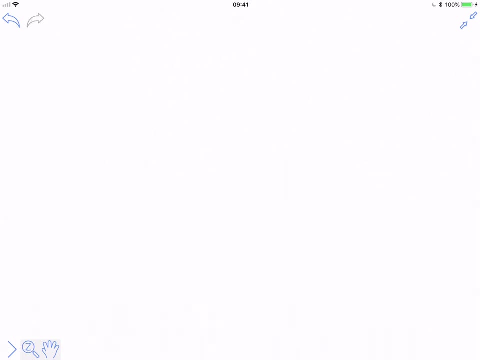 you guys have already read. if you've read the reading for today, you've already read how we proceed with the mechanics. What are we going to do In order to make sure that all those variables are zero at the moments that we are looking? 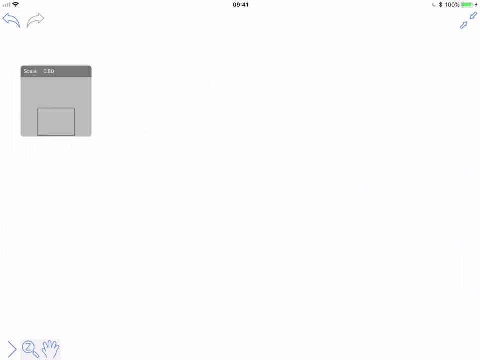 at them, or where we start. we are going to make new variables. So for every single variable that we have, let's say: this is now u1.. Now let's say u1ças non-zero steady-state value, and we can just say that that non-zero steady-state. 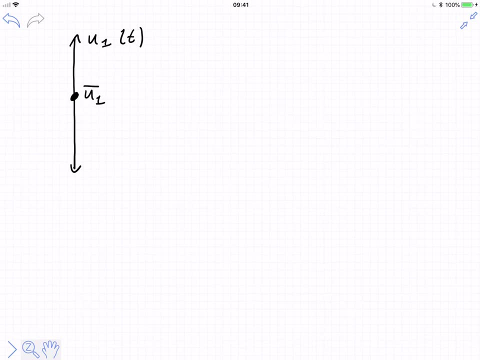 value is u1 bar. What we're going to do is we're going to introduce a deviation variable version of that, and I just want to actually match exactly the notation of the textbook here. Please note that the textbook there isn't 100% agreement. 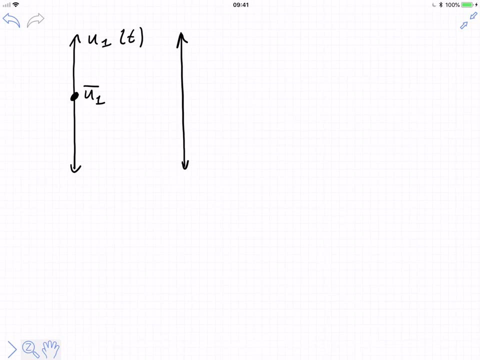 between all the different ways of expressing this idea. Some people use hats for the deviation variables. The textbook uses primes for the deviation variables. Just be clear in your mind. there's a limited amount of notation available for writing down things and I know that you've seen primes being 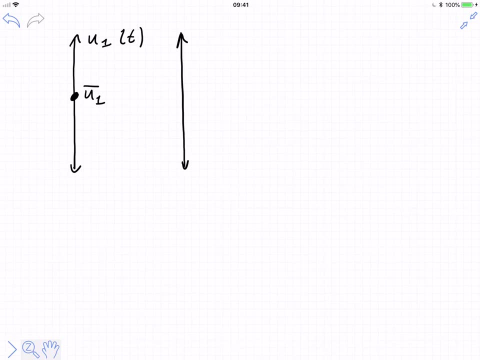 used before for derivatives. So just remember, in this subject I will basically never use a prime to indicate derivative. Just to be clear what I mean with prime. this is u prime, That little dash over there is called a prime. So I will never, ever ever, in the entire space of this course, ever use 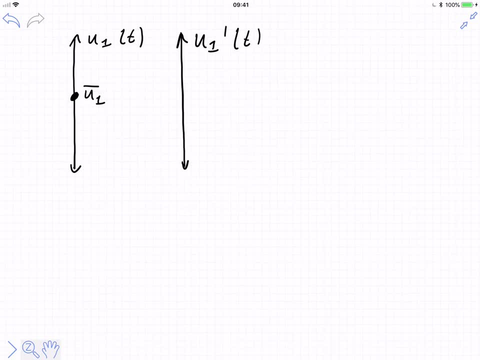 that notation to indicate a prime derivative. I will always use it, at the very most to indicate deviation variables. And so what exactly is a deviation variable? It's a variable where I have taken that exact same place, the same value, and I have made that zero. So I've just 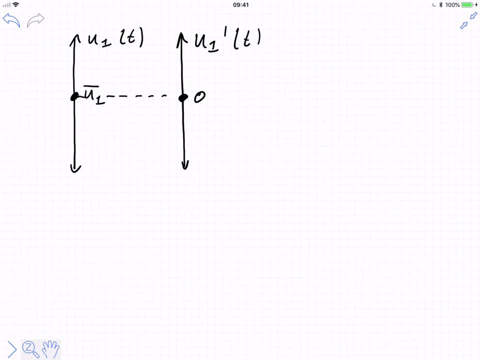 relabeled these axes, right, So you guys are aware of you've seen shifting axes before, right, So you've seen this idea. Now I've just done this on a one dimensional axis like this, just because in many cases we like having the x-axis. 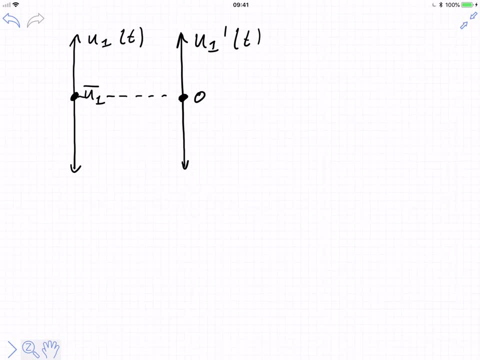 in this subject, The x-axis in this subject being time, right. But if I were reading this on a graph, let's say I was seeing something that was varying over time like this, right, You can imagine that I could have just used. this is very similar to the. 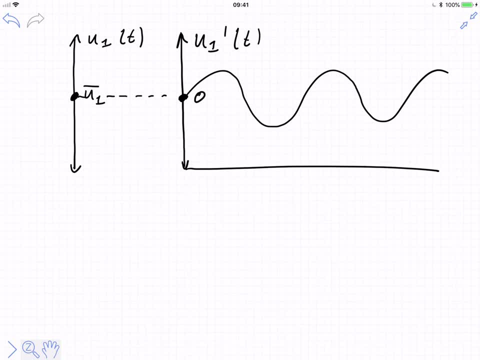 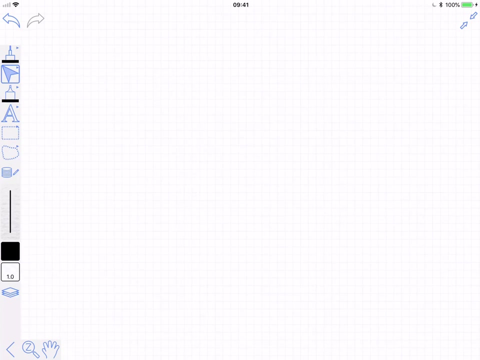 kind of translation that you do between Kelvin and Celsius, right? So imagine that I've got a time varying temperature measurement like this, okay, And imagine that stuff isn't freezing or anything, but for some reason we've kind of got the cytosol motion around zero Celsius. You agree that at the same moment where the Celsius 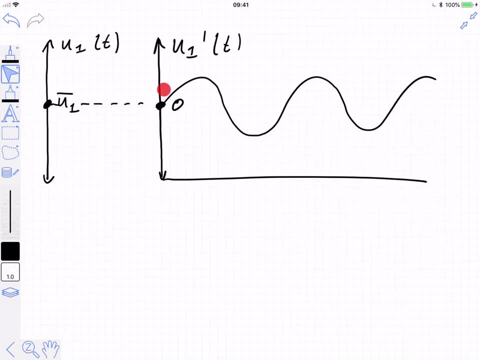 temperature. at the same moment, where the Celsius temperature is zero, the Kelvin temperature will be 273, right? And so there's this relationship between these two axes, between the Celsius scale and the Kelvin scale, where they behave in exactly the same way. they. 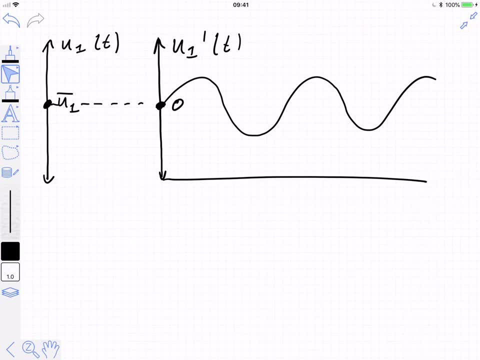 just have different values. They don't have the same values, They just have different zeros. okay, So deviation variables are exactly the same kind of idea. We've got one set of variables which are the original variables, and they are the variables that we wrote down originally when we wrote down the model, right? We? 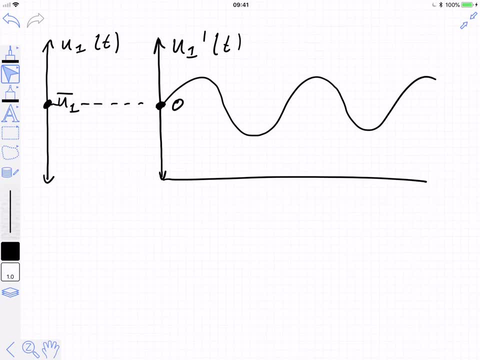 measured a length from somewhere, or we measured a temperature, or we measured a pressure or something like that, and those were just the original variables And now we are going to introduce- you can imagine, almost like different units, right? And these units, just like the Celsius scale and the Kelvin scale, 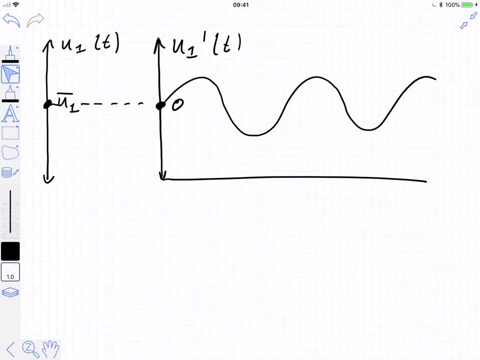 are shifted with respect to one another by this constant. The original variables and the deviation variables are going to be shifted with respect to one another in a very special way. They are going to be shifted so that the steady state values of the variables are zero in the deviation set of axes right. 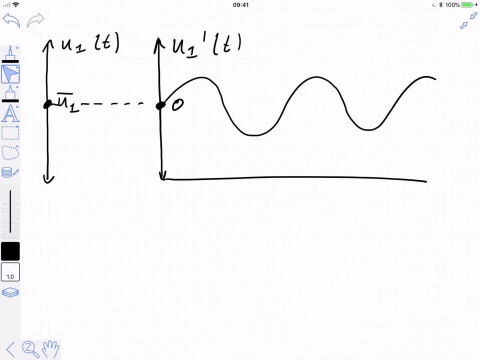 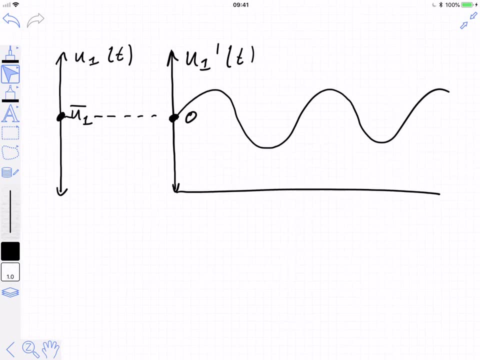 So now, how can we capture the math behind this Very, very simple right? It's super clear, It's very simple that U, U prime is just going to be the same as U1, except that it's going to have the deviation or the original point, whatever the steady state value of 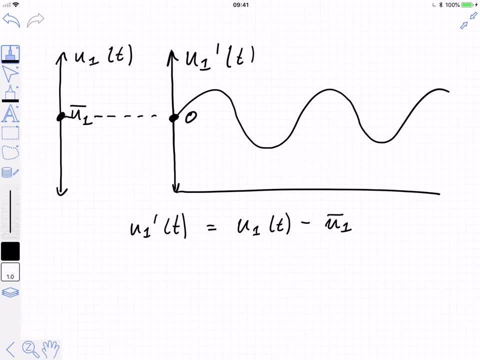 U1 was subtracted. I know this is a concept that takes a while, so I'll just just cover to sink in. The mechanics are actually a lot easier to understand than the concept, I think, because from a mechanics point of view, all you do is you say: I am going to introduce these. 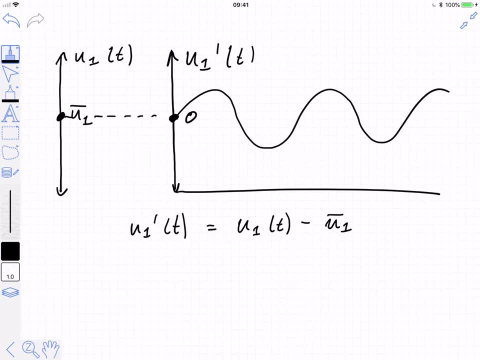 variables and then moving to the new variable simply involves a little bit of algebra and substitution. right, Because you then say: if this is the definition of the deviation variables, right, And this, we'll introduce this. this is exactly the same definition as in the textbook. 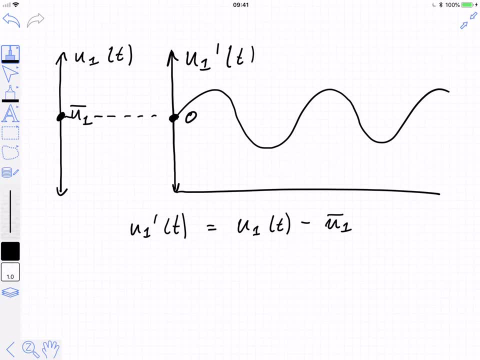 you'll see this in equation 3.4 in the textbook they introduce this. they use even like a little triangle over there to kind of say this is like what it is by definition, right, So it's a deviation variable and you can kind of imagine that this is like a placeholder I've used specifically. 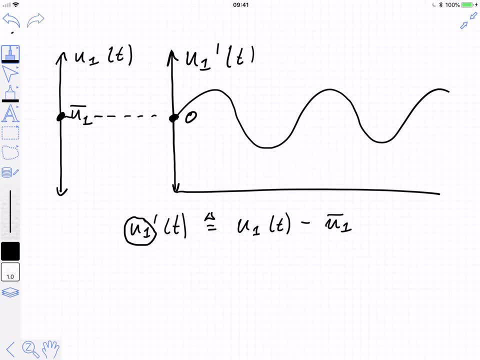 u1 now, but that obviously could be anything, right, It could be an x, it could be a y, it could be just what you want, and we'll just use this notation. we'll say: there's a prime there, so it's. 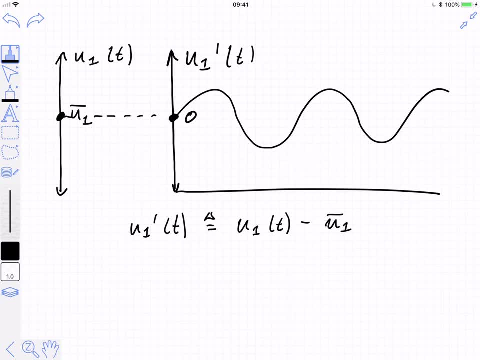 a deviation variable And we've taken steps to make sure that that now is zero at the initial condition or steady state. Now you'll also hear me say initial condition and steady state approximately interchangeably, because one of the assumptions that we'll be making when we solve these: 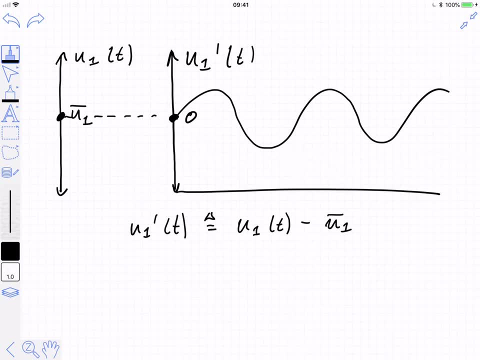 differential equations is that the initial state is steady state. So we will not really be solving lots of differential equations where there's a transient state, For instance. things that we are not able to solve easily with our approach is something like a ball that is falling right. If time zero involves that ball already being in motion. 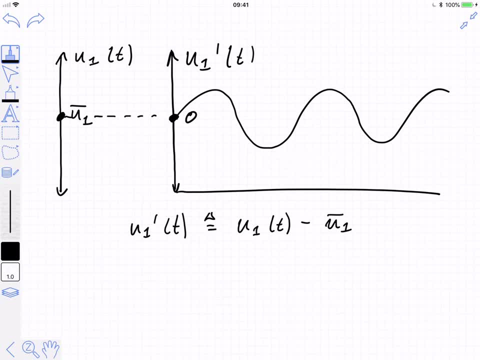 some of the states are not zero and some of the state derivatives are not zero and therefore our approach will fail because of that. In most of our systems it's possible to make steady state happen, And so you've seen already, when we did the simulation of the 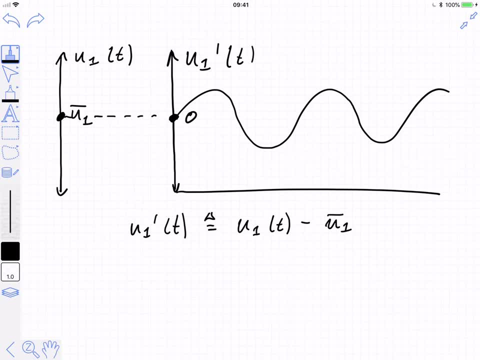 CSDR two weeks ago. we started out by solving for the steady state first, So we said, okay, let's just start where everything's fine and nothing's happening, and then we'll go from there. What would happen if the system were then disturbed? over time, It makes all of 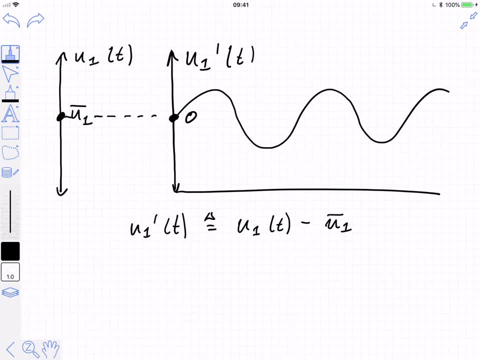 our stuff a lot easier to deal with. So this bar will always be used in our subject to indicate steady state, And what that means is, if I substitute the barred versions of variables into a differential equation, I'm guaranteed to get a zero derivative. And that's a very important step because we want 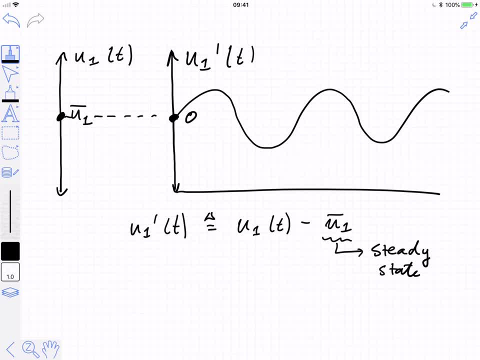 our steady state So effectively. that's the definition of steady state, right? The definition of steady state is: all of the derivatives are equal to zero. all the time derivatives are equal to zero. So that's the first step. The second step is to get a zero derivative And the third step is to get a. 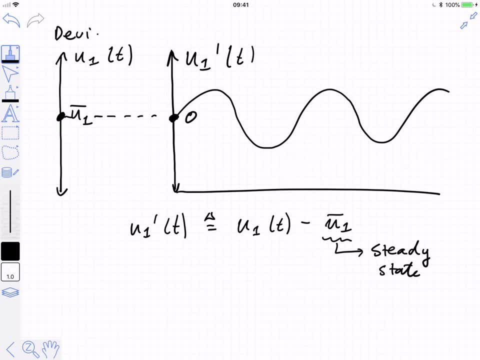 zero derivative. So the first step this is deviation variables. Now, a consequence of using deviation variables is that once we've done this, all the constant terms in our differential equations become zero. So we may originally have had constant terms, right? If we just wrote down some kind of equation, there may have been a constant. 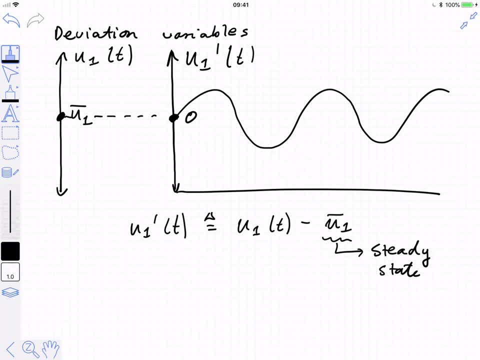 term, But because when we substitute our deviation variables in, we know that the constants will all cancel out, so that the derivative is zero when the states are equal to the deviation variables. We make that happen by design And you can see how that plays out in the. 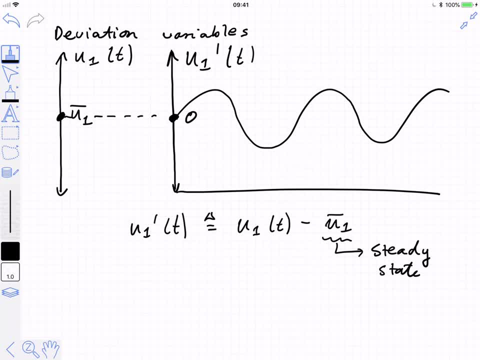 example, in 3.1.. But I feel like this: having this kind of a graphical intuition about deviation variables rather than just algebra, makes them easier to apply, But the mechanics are the same. So we're going to have to do a little bit more of that. So we're going to have to do a little bit more of that. 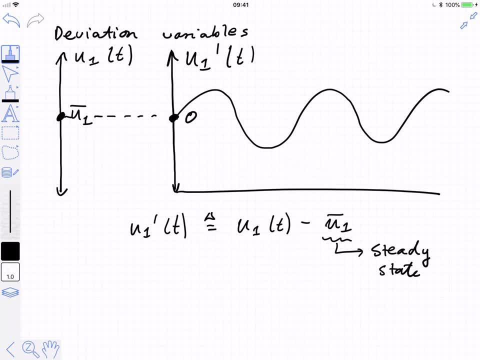 I find it really the easiest to say: I will now, if I want to get away from my original variables, just solve for my original variable in that equation. So in other words, u1.. And I'm going to drop the t's here just to make the notation a little bit simpler. I recommend: 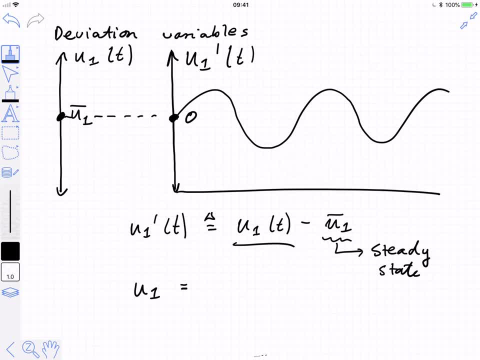 that while you guys are getting started, it is useful to kind of keep the t's in there, just to remind yourself which things are constant and which things are changing with time. I do not subtract any marks if you don't put the t's there. 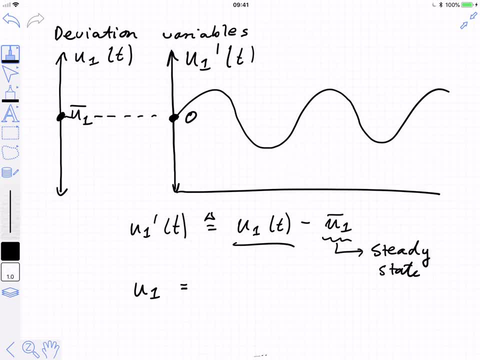 Sorry. So it is a little bit faster to write And it's not that hard For most of our models. it's not that hard to keep track in your mind of which things are time-varying things and which things are not time-varying things, At least if you've written down your model. 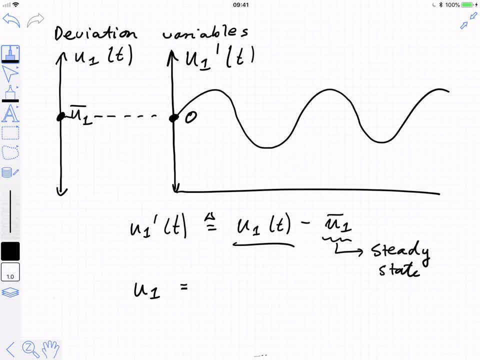 in the form that I recommend. you've made a list of the parameters anyway, And those will be all the time-varying things, So we'll write down here: u is equal to u1 prime plus u bar, And this is effectively the mechanics or the algebra that we will need to do to get. 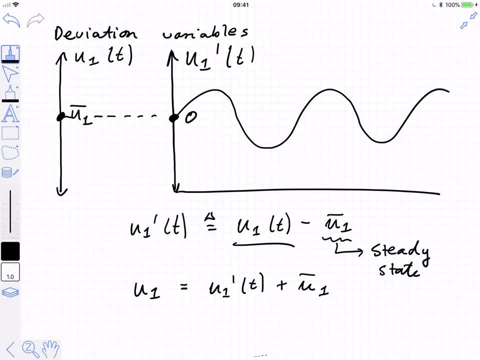 our equations which started off in the real world, into deviation variable form. We'll just substitute all the real variables for their deviation variable form plus u bar, And so I think this form makes it easier to understand the shift relationship, And so this form makes the algebra easier, because then it's just substitution. 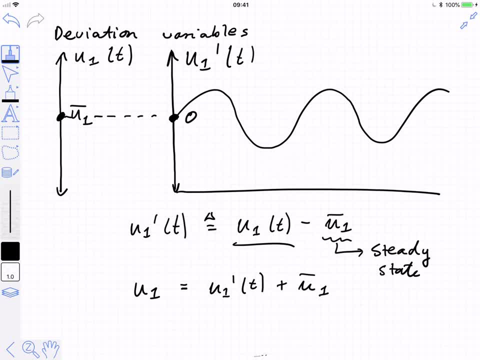 So that's deviation variables, The other thing that we'll do. so we'll do these two things. This is not an approximation, This is just the shift of axis And we lose no accuracy by this substitution. You can see, that's straight up good math. I'm not like. there's no squiggly. 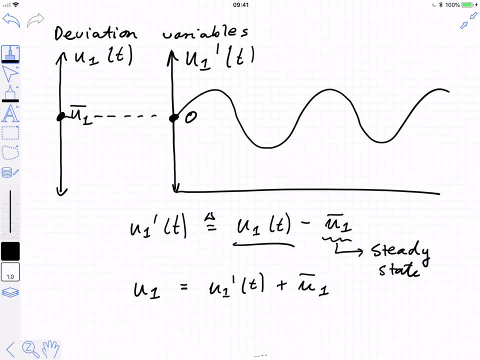 equals or anything like that. At this point, I have not yet lost precision. I've only made it easier to see. Now I'm going to show you where steady state is. Steady state is where all my variables are zero. Now, now that I've done this substitution, I will end up with a model in terms of u1 prime. 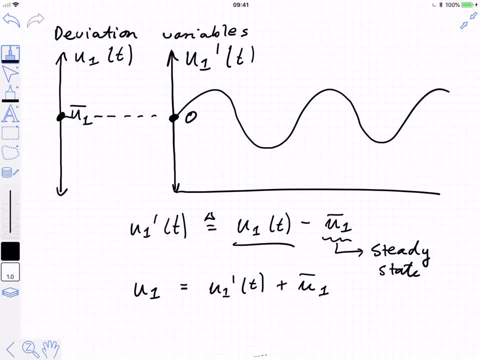 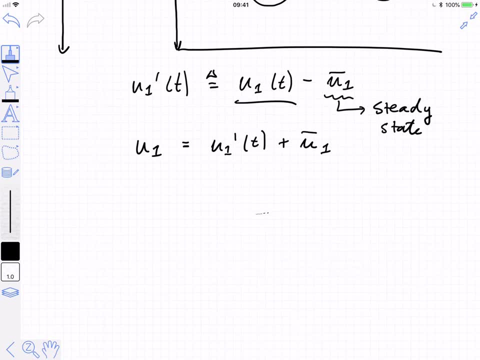 And that model will have this characteristic that when I solve for steady state, the steady state will be equal to zero. All the? u primes are equal to zero at the steady state. The second thing that we'll do is an approximation, And this is linearization. 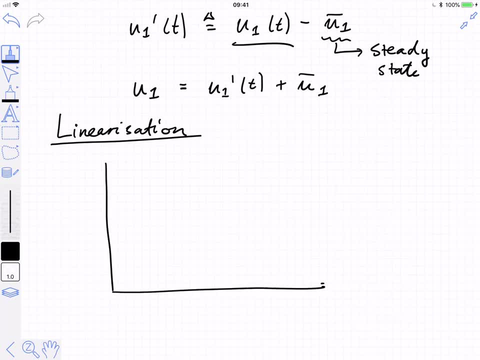 And what we'll be doing and now notice here that the x axis here is not time. We are going to take a variable. Well, let's say, let's say we take this function And we're going to approximate it at some point. Ah, probably easier this way around. Okay, Please note. 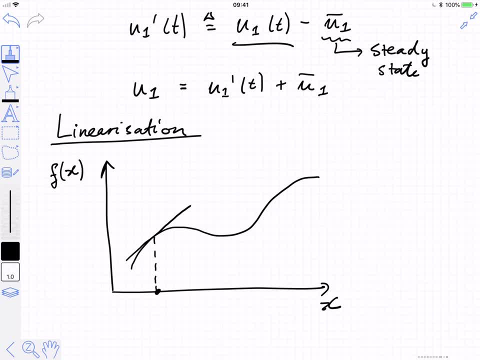 we don't do this for functions of time, All right. So be very clear. It's easy to imagine, because we're going to be drawing mostly graphs where the x axis is time. it's easy to get confused. Okay, I'm going to have to do this for functions of time as well. 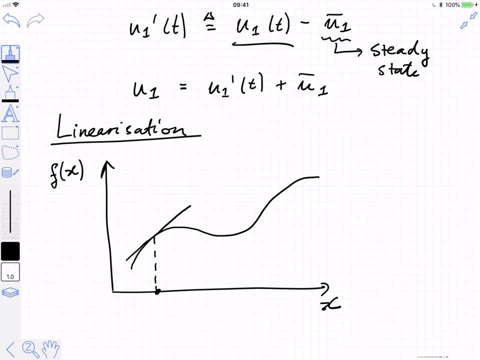 We don't do this ever for functions of time. In other words, we never do this if this axis here is time, right, We don't do it like that. So these are for nonlinear terms, where we are trying to capture the behavior of that term. 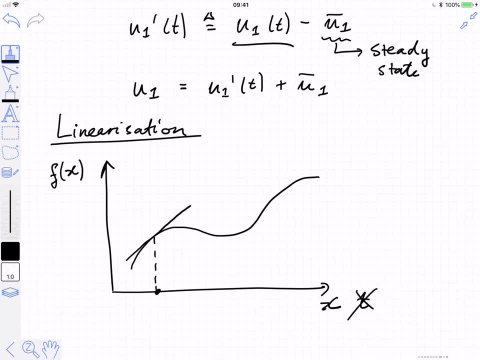 And what we're going to do is a first order Taylor series expansion. So we're going to take at that point, we're going to take the derivative and we're basically going to say: let's imagine that the whole of the function is described by the behavior of that tangent line. 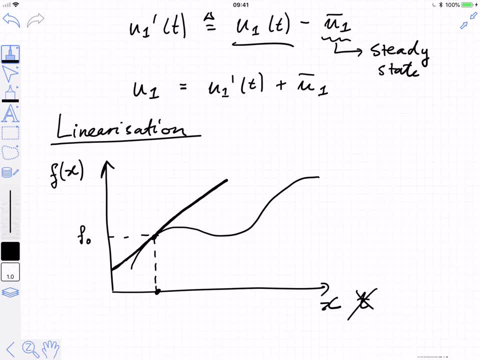 So what is a first order? Taylor series expansion? It is simply the equation for that, For that line, right? So we're going to say: at x0,, at x0, the function value is f0. And the slope of that tangent line is df. dx at my hands, go too fast- dx at x0. 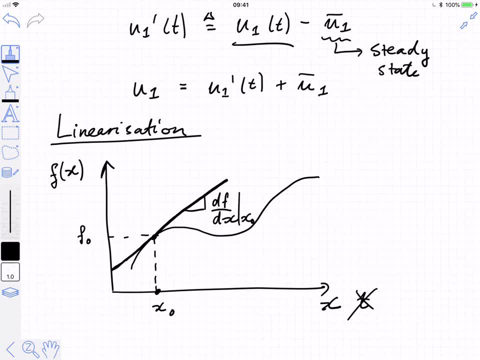 And so the equation of that line, we're going to say: we're going to approximate that f of x. Now, this is a true approximation. So I'm going to use my little approximation squiggles And I'm going to say: right, it's just going to be f0 plus. and I'm writing it in this form to highlight this: Taylor series expansion nature: right. 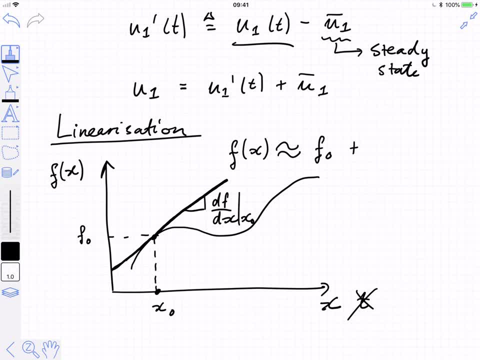 So at this point, without the plus, I would have a A zeroth order. Taylor series expansion right. So this is the. This would be having f of x equal to the value of f. at the point that I'm doing, my approximation would be a zero order. 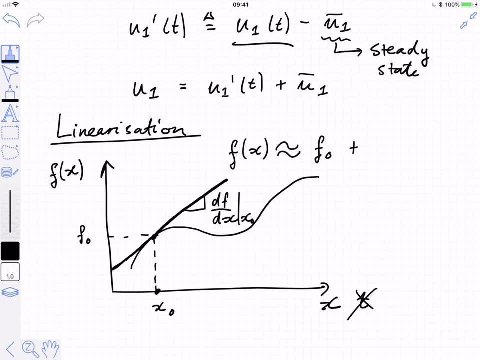 And then I'll add the linear term. And you'll remember that the Taylor series has this wonderful effect that I can just add all the higher order term. right, I can start with a zero order term. If I want another piece of precision, I can add a linear term. 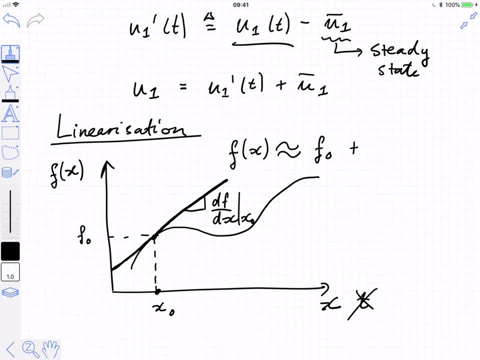 If I want more precision, I can add. If I want more precision, I can add a quadratic term. If I want more precision, I can add a third order term and so on, And I don't have to recalculate all the previous coefficients. 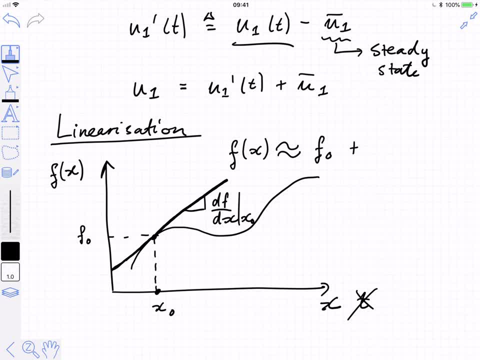 I just calculate the coefficients as I go, And so now I need that slope, And so this will be df, dx at x0.. And in order to make that coefficient usable in a nice way, I just add that extra linear term, which we will now see. 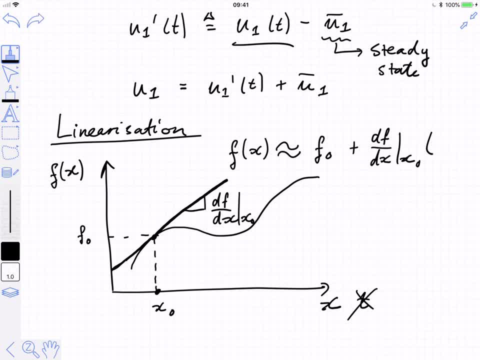 is x minus x0.. And if you're paying careful attention, you'll notice that this looks very much like the definition of x prime. Right, It's the original variable minus some point at which we are doing the approximation. Now these two things, then they work together. 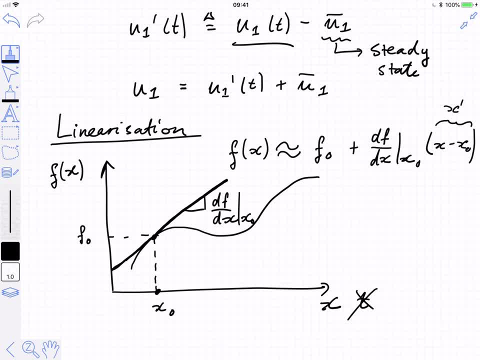 If we do a straight linearization, we find the deviation variables therefore kind of jumping out very naturally from our approximation, Right? Because we see, oh yes, well, whenever I do this kind of linearization, I will always end up with this: coefficient times a, x minus x0 term. 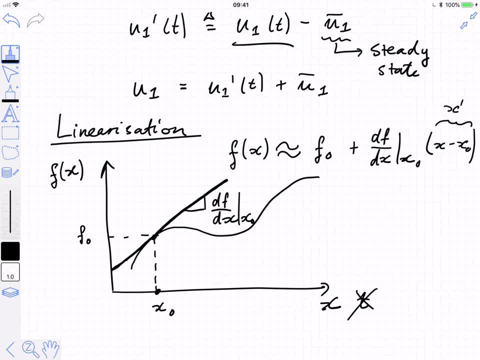 And for the same money we could have called that x0, x bar And it would be the same operation. So these two operations together, linearizing all the nonlinear terms, and you know you don't have to specifically linearize the nonlinear terms. 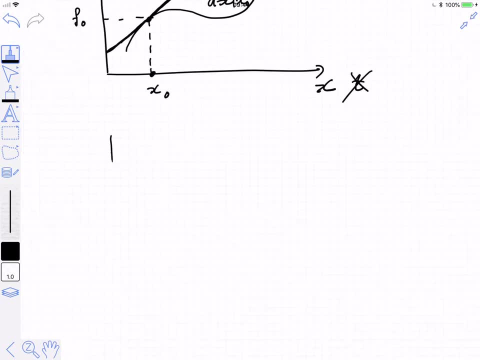 because I just want to show you that if the original equation were linear, to start with right, So let's say this was the original equation, It doesn't matter where I build my approximation, If that slope is m right, Right, I'll always recover. 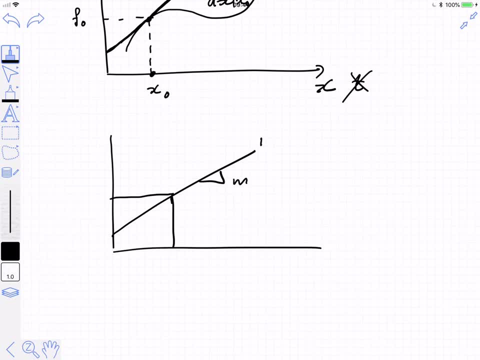 So let's say this was mx plus c, Right? Let's just imagine I want to build a linear approximation of that relationship. What will I find? I will find that at my point of approximation. so let's say x0 over here. 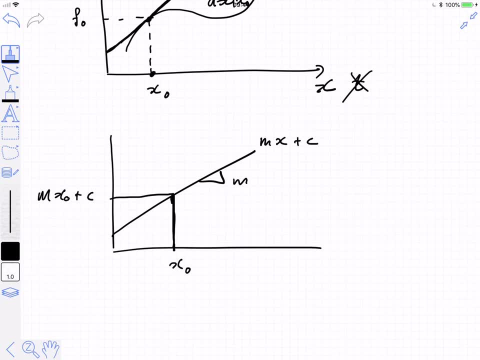 I will find mx0 plus c as the function value at that point Right. And if I'm doing my linear approximation, I'll have mx0 plus c plus my linear term, And that linear term, remember, the slope will just be straight m right. 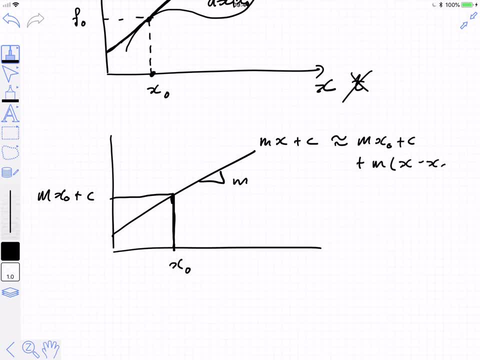 It will be m times x minus x0. And so I don't have to specifically avoid this. If I were writing a computer program to do this, I would just do it on all the terms. If you're doing it by hand, you can save yourself just this little time. 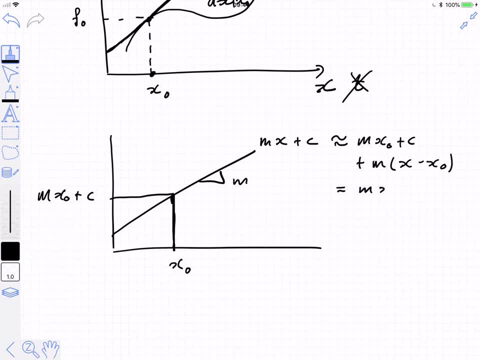 because obviously that then will end up being again mx plus c. Okay, So applying linear approximation to something that is already linear leaves it unchanged. That should be an unsurprising result, but at least we know that we will never make a mistake. 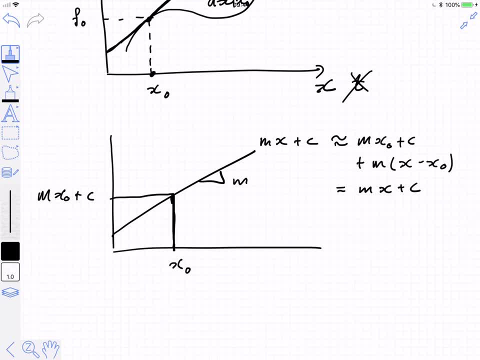 if we by accident linearize a term that was actually linear to begin with. So it's perfectly fine to just say: well, we just linearized the entire equation In terms of the mechanics. obviously you write less if there's just one nonlinear term. 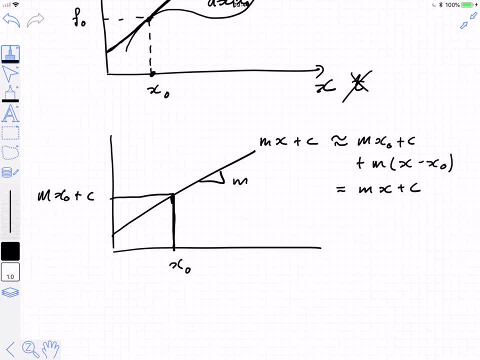 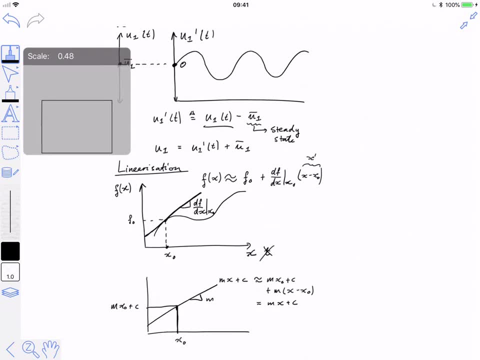 You write less if you can just find that one term and just do that approximation. So these are the two steps Now I will. tomorrow we'll go through a full example, but I just wanted to kind of give you some visuals here. 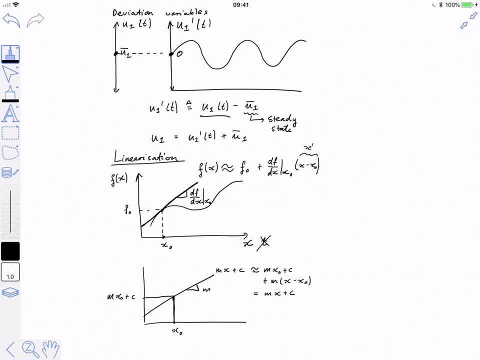 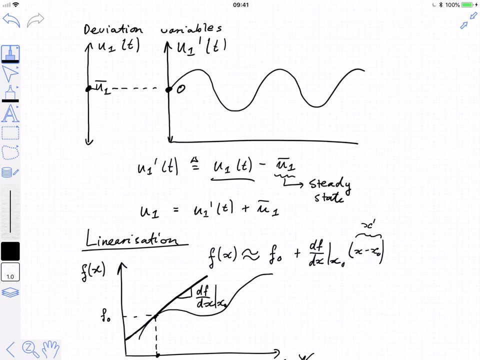 because the textbook is a bit thin on visuals in terms of explaining the process. It just says, well, we do this, and kind of, here's how we do it. I also want to give you some examples, So I'm going to take a little bit of time while I've got you in a place where I can show you a computer screen. 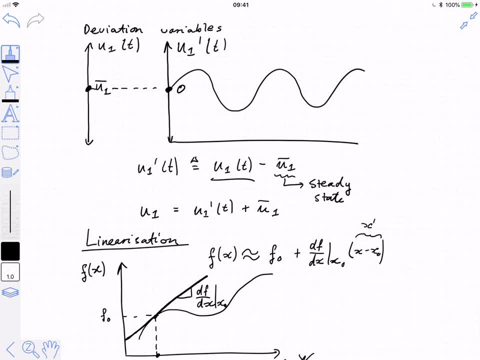 to show you that many of these steps we can actually do using the computer as well. So, because we're and remember you will be writing with a computer in front of you Now, if a lot of you are perhaps not as fluent as you perhaps would like to be, with interesting derivatives. 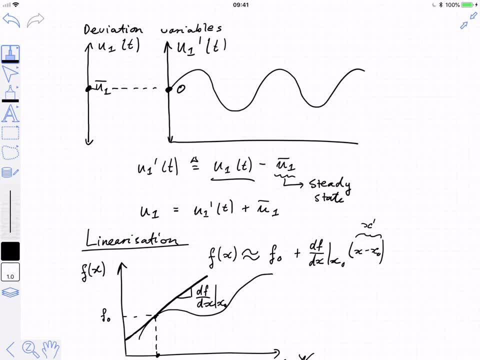 I know that, for instance, I am terrible at like memorizing interesting derivatives, you know. so who can tell me quickly what the derivative of x times log of x is? You know, like who knows, You're going to have to kind of go through quite a lot of steps to get there, right.